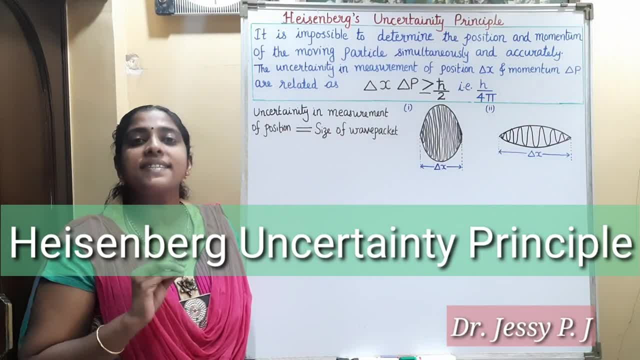 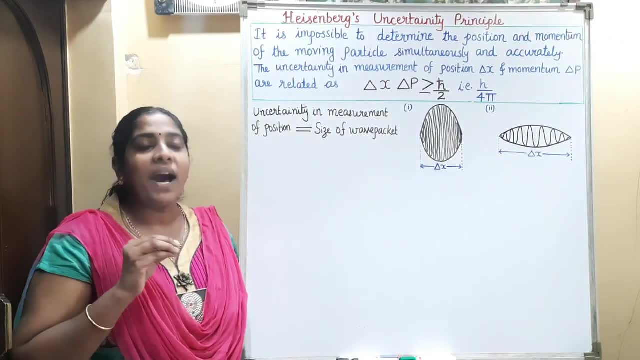 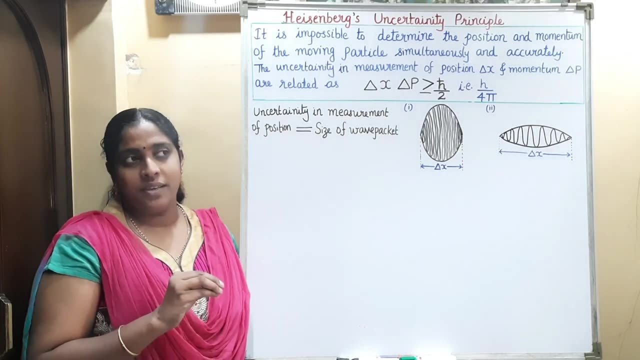 Hi all. today we can discuss about Heisenberg's uncertainty principle In classical mechanics when we study the motion of objects, when a particle is moving, the position and momentum of that moving particle can be found out accurately, Because if we know the initial position and velocity after a given time, we can find out. 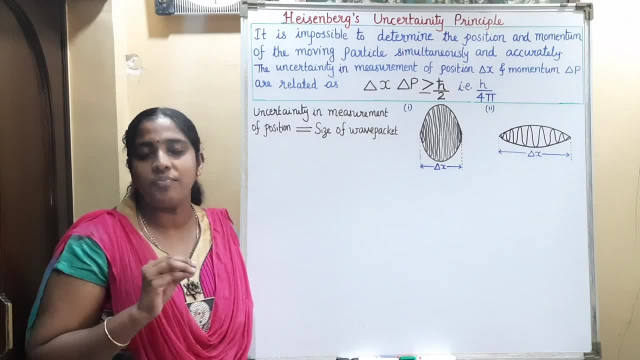 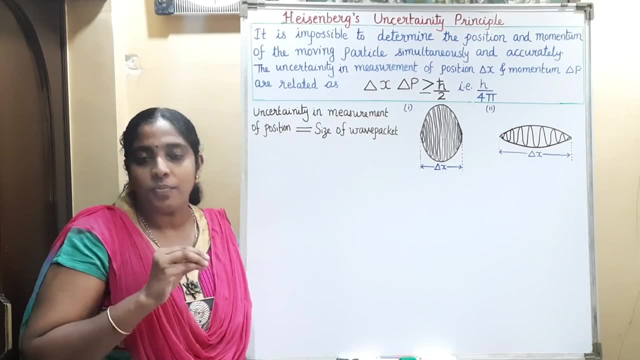 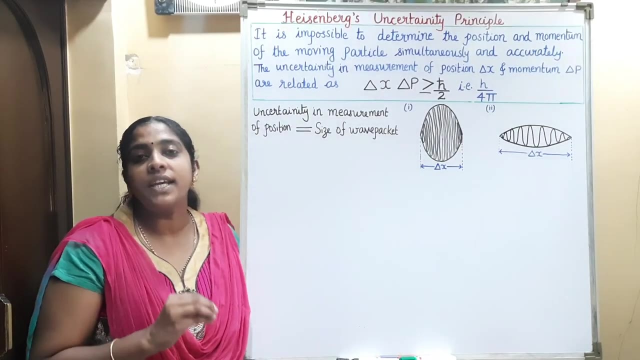 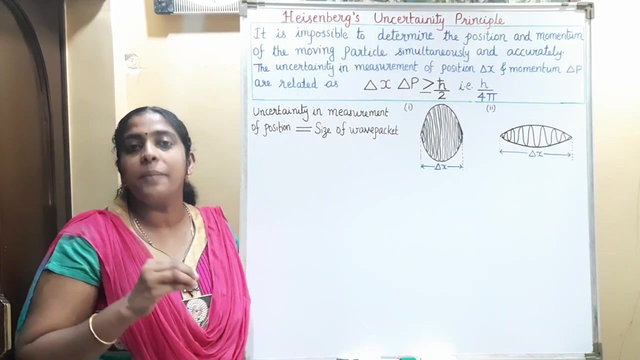 the position and momentum using Newton's equations of motions. But when we consider an atomic particle, an electron or proton is moving. we cannot find out the position and momentum accurately Because when we consider an atomic particle, a matter wave is associated with that, and Schrodinger postulated that a microparticle is equivalent to a wave packet. So when the 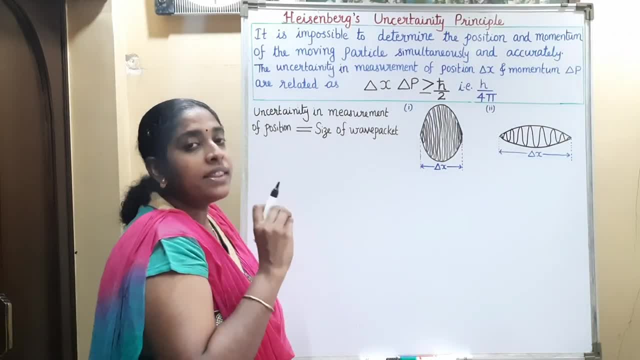 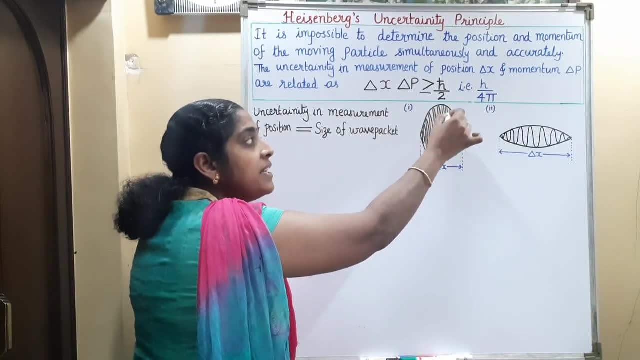 particle is moving, the position and momentum of that particle can be found out accurately. If a wave packet is moving, then where will be the exact position of that moving particle? That particle can be anywhere within this wave packet, but we don't know exactly where will be. 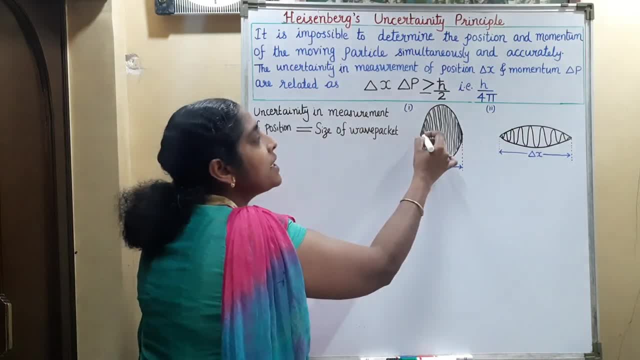 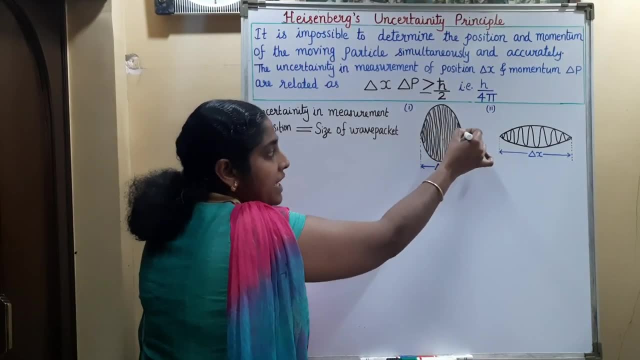 the position of that particle. We can say that the probability of finding the particle will be maximum at the center of this wave packet and that probability of finding the particle will decrease at the end, but we don't know exactly where will be the position. 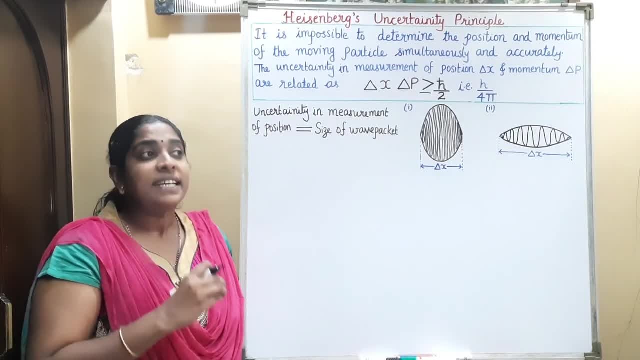 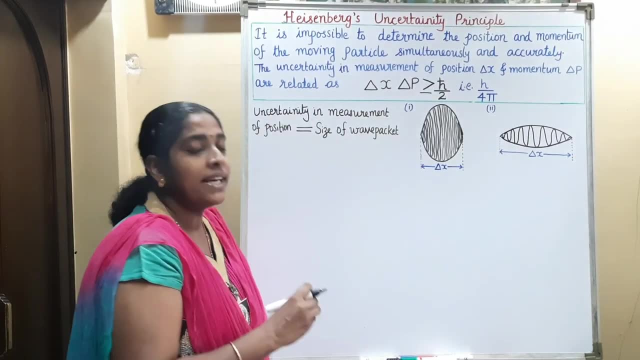 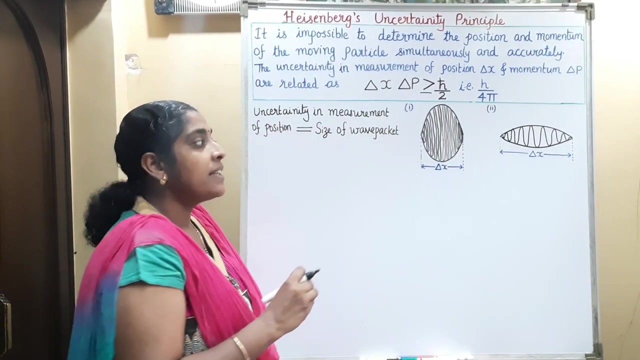 That means there is an uncertainty in determining the position of that particle within the wave packet. Then what will be the uncertainty in determining the position of that particle within the wave packet? That will be equal to the size of the wave packet If delta x is the 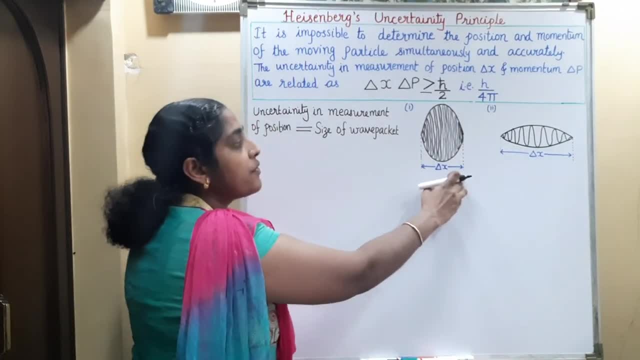 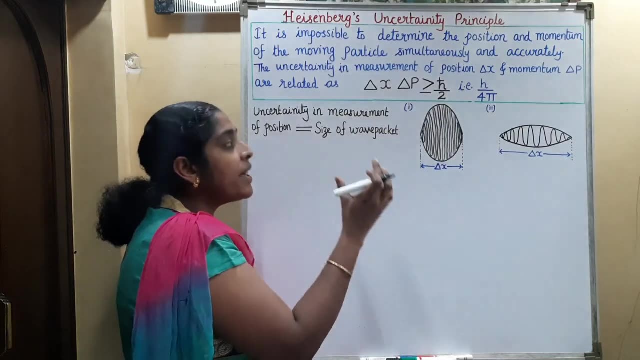 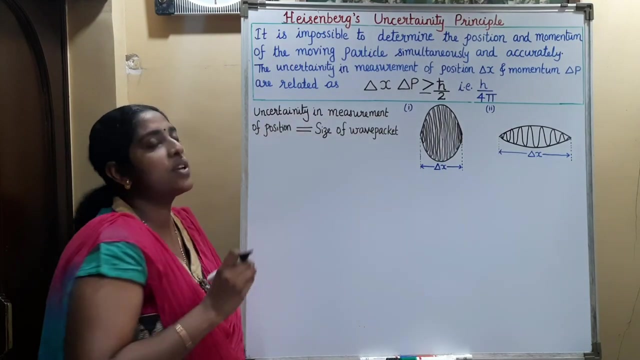 width of the wave packet, that is, the linear spread of the wave packet. the maximum uncertainty in determining the position of that particle within the wave packet will be equivalent to this. delta x, That is, uncertainty in measurement of position, will be equal to the size of the wave. 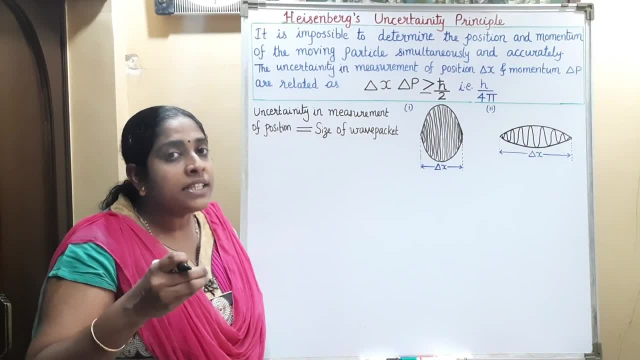 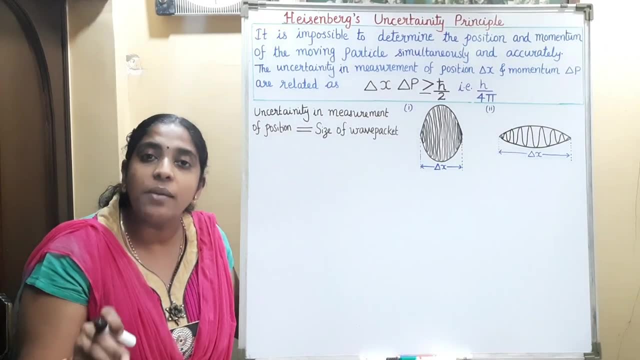 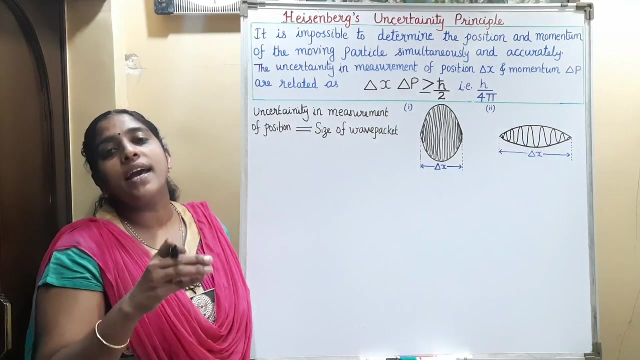 packet. If there is an uncertainty in determining the position of that particle, correspondingly there will be an uncertainty in determining the momentum also. That means, along with an uncertainty in the determination of position, there will be an uncertainty in determining the momentum also. We can see two wave packets here. The first, 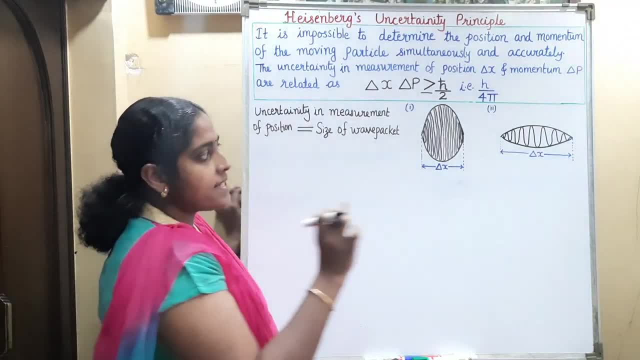 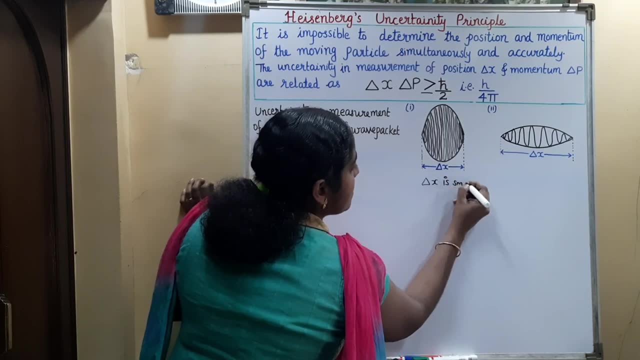 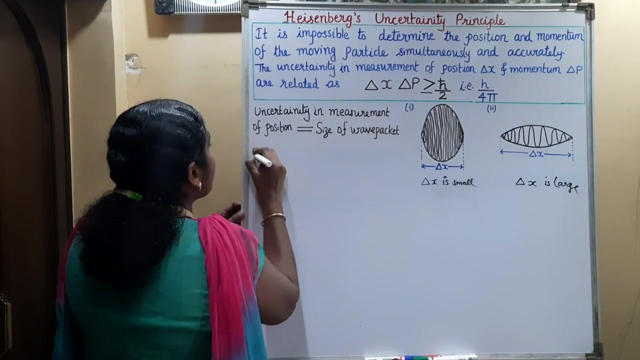 wave packet the width is small. Second wave packet is a wider wave packet. That is here the linear spread of the wave packet. delta x is small, whereas here delta x is large. That is, the first wave packet is a narrow wave packet and the second wave packet is: 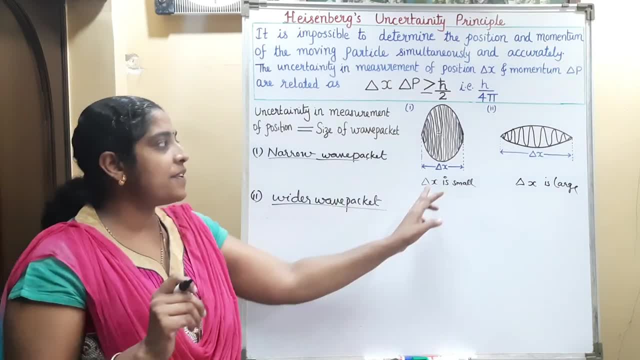 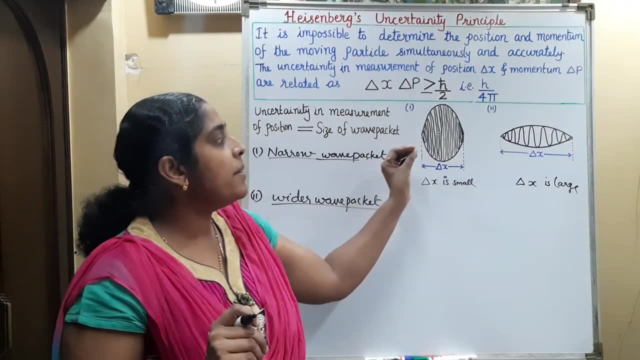 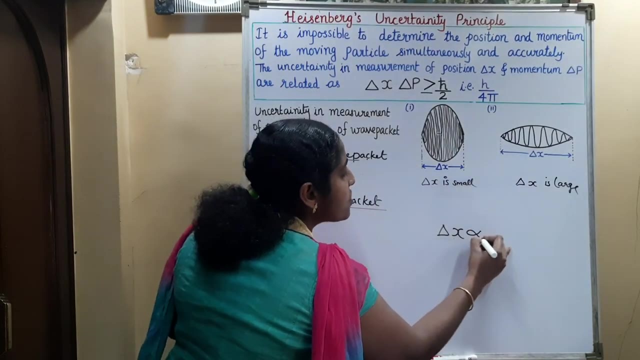 a wider wave packet. So in the first narrow wave packet delta x is small. To construct the narrow wave packet there will be more. number of verbs are required within the wave packet, That is, delta x is inversely proportional to delta k. K is propagation constant, Delta k is a term corresponding. 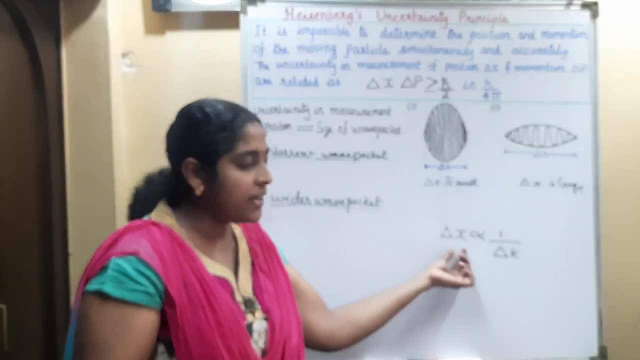 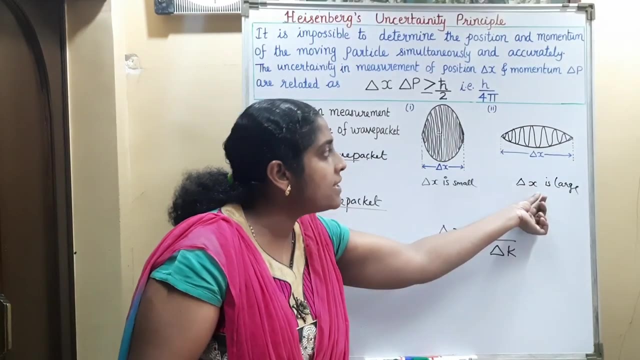 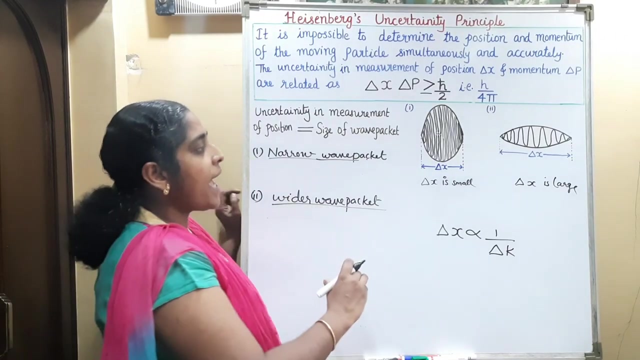 to the wave number. To have a narrow wave packet- small delta x, more number of verbs are to be included within the wave packet, And for the wider wave packet the number of verbs are less because delta x is large and number of verbs are less. So in the narrow wave packet there are more. 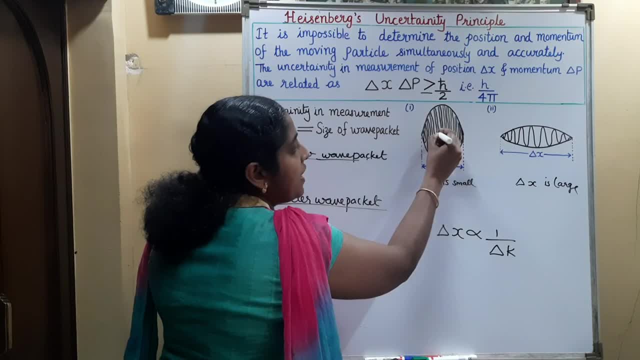 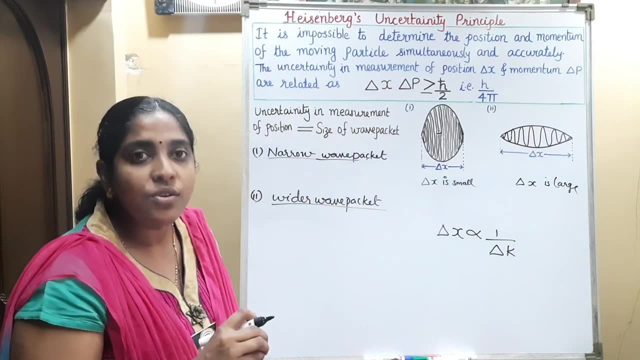 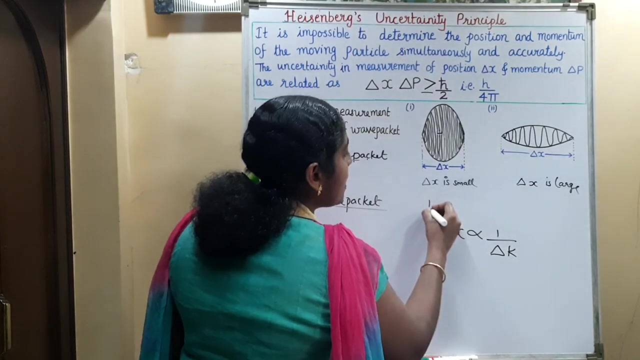 number of verbs. So the determination of wavelength within this way packet is difficult. If there is an uncertainty in the determination of wavelength, there will be an uncertainty in the determination of momentum also, Because is equal to h by lambda. if there is an uncertainty in the lambda, there will be an uncertainty in the. 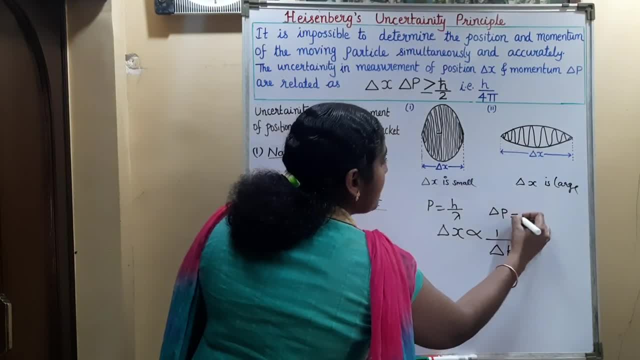 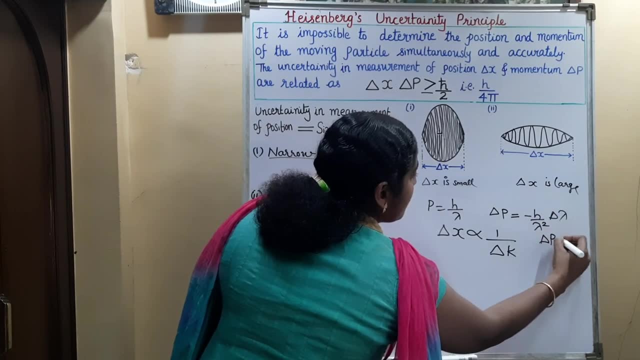 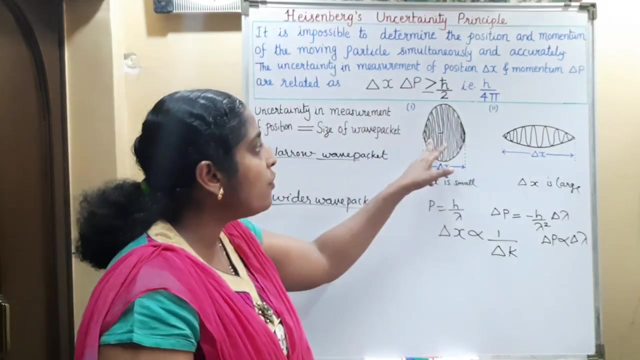 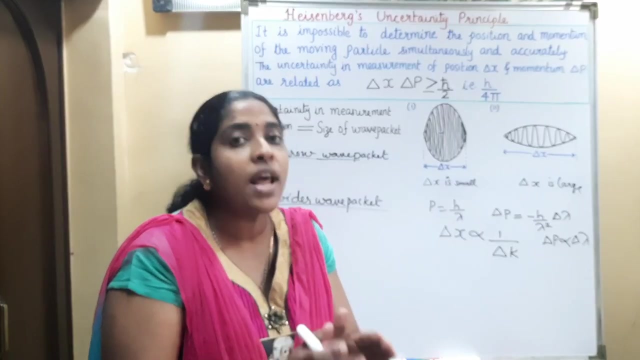 momentum, because that uncertainty in the momentum, delta p will be equal to minus h by lambda square delta. lambda that is delta p. uncertainty in the momentum determination is directly proportional to the uncertainty in the wavelength determination. so in the narrow way, packet the world, there are more number of verbs and uncertainty in finding the wavelength will be more and correspondingly, 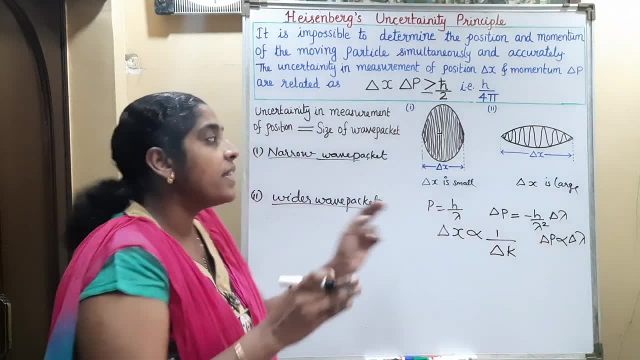 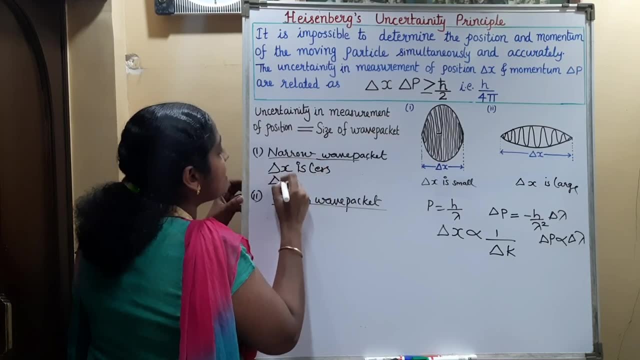 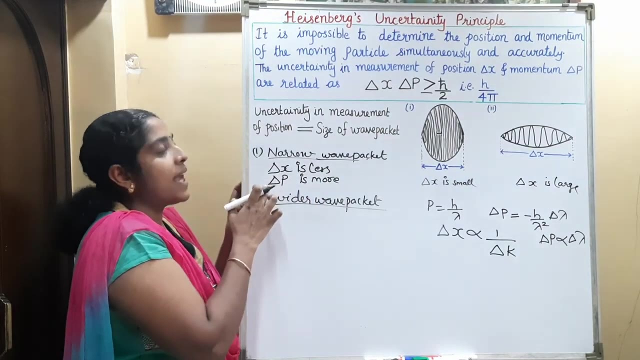 the uncertainty in finding the momentum will be more. that is in the narrow way. packet delta x is less, but this delta p is more. what is this delta x? uncertainty in finding the position will be less, but uncertainty in finding the momentum will be more. and what about in the 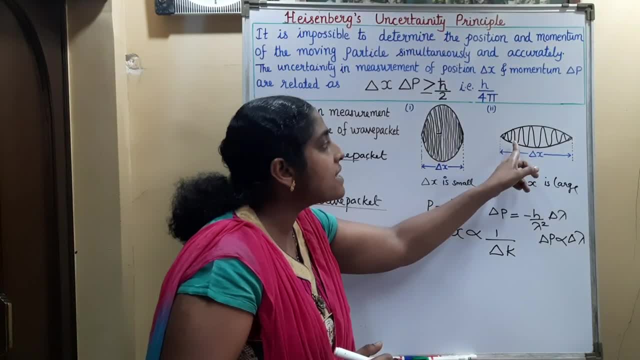 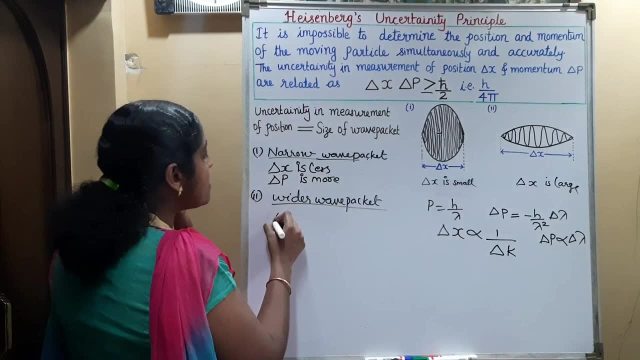 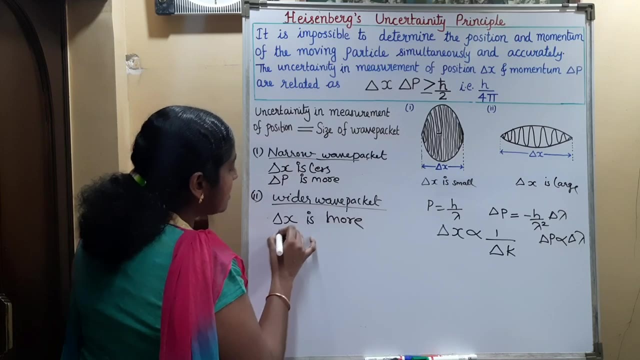 wider way packet In the wider way packet In the wider way packet. Why wave packet? the uncertainty in finding the position is large due to this large linear spread. that means this uncertainty in finding the position is more, but this uncertainty in finding the momentum will be less, because here it is. 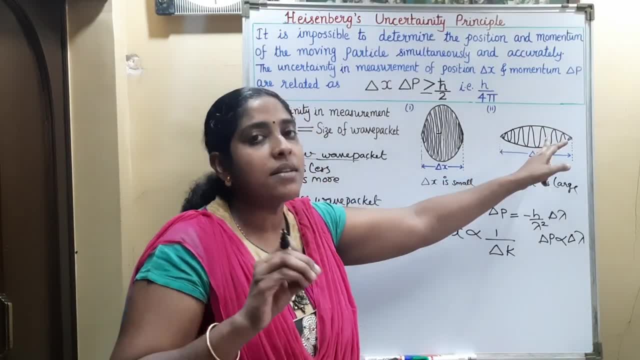 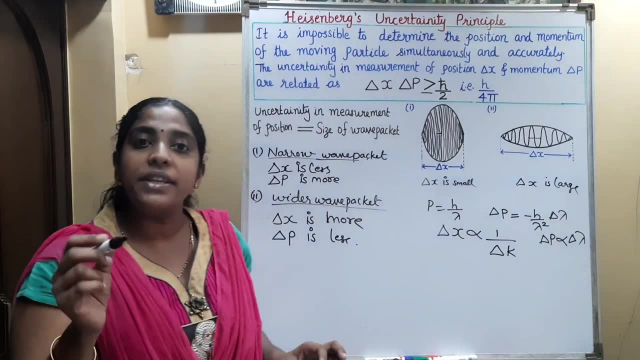 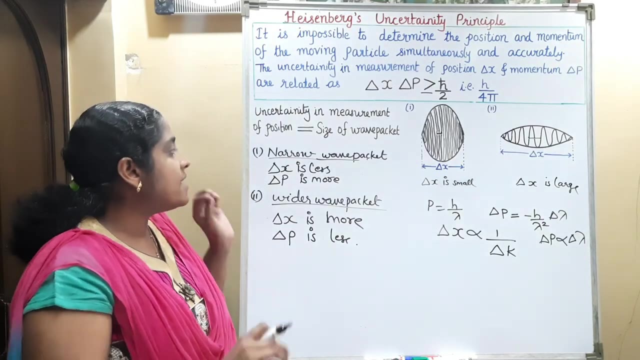 clear that in wider wave packet there are less number of waves, so the determination of wavelength is easy. so the determination of momentum will be easy and the uncertainty in the finding the momentum of that particle will be less. that is when the uncertainty in finding the position is small. 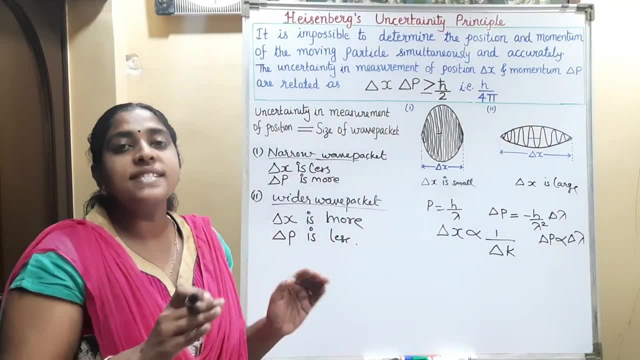 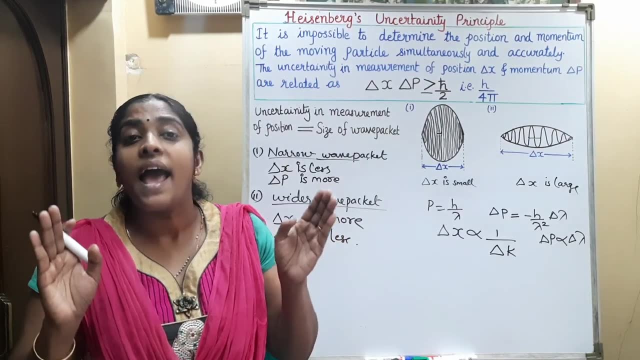 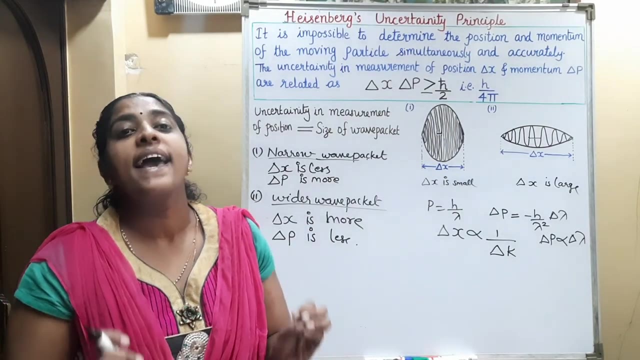 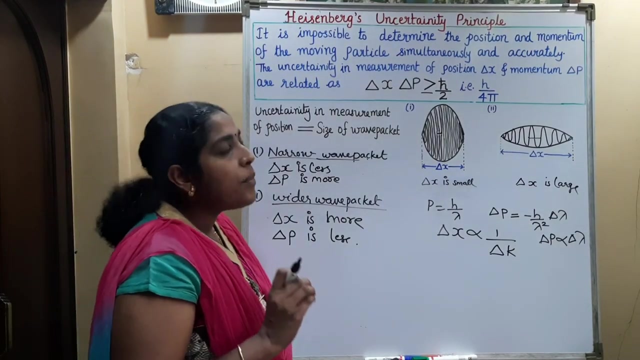 uncertainty in finding the momentum is more, that is, simultaneously we cannot find the position and momentum of a moving particle accurately. so this was significant suggested by heisenberg, and this principle is known as heisenberg's uncertainty principle. so heisenberg uncertainty principle states that it is impossible to determine the position and 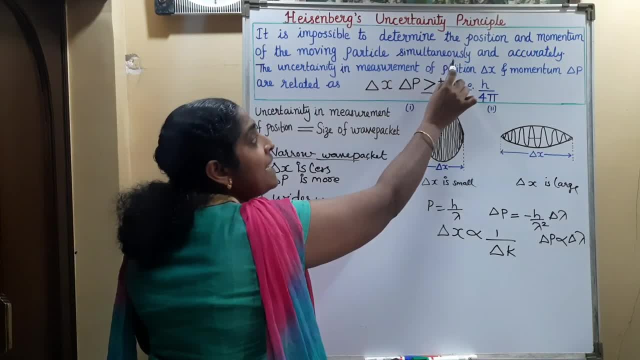 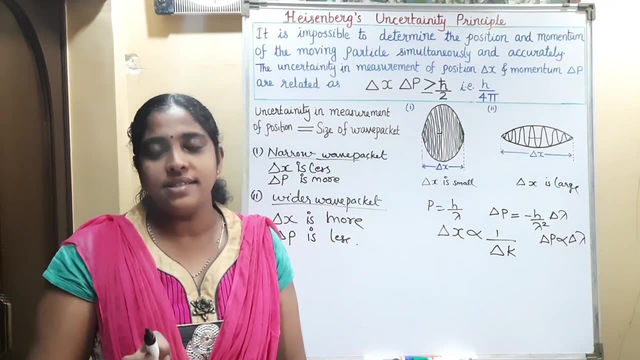 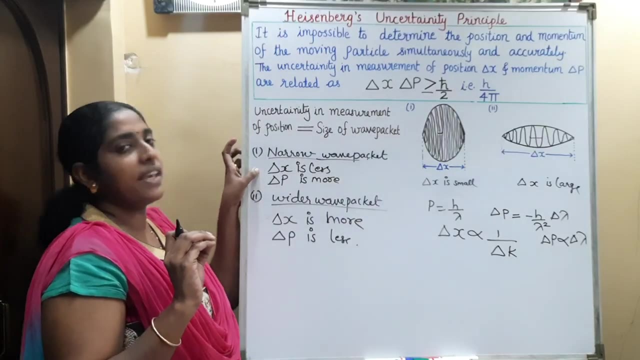 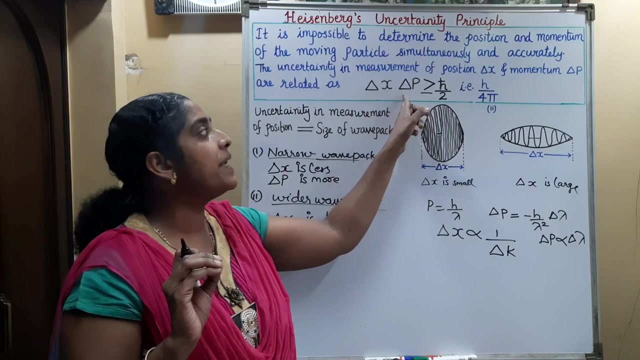 momentum of a moving particle simultaneously and accurately. we cannot find out the position and momentum accurately at the same and simultaneously and heisenberg suggested this. uncertainty in finding the position, delta x and uncertainty in finding the momentum delta p is related, as delta x, delta p greater or equal to h cross by 2. that is the 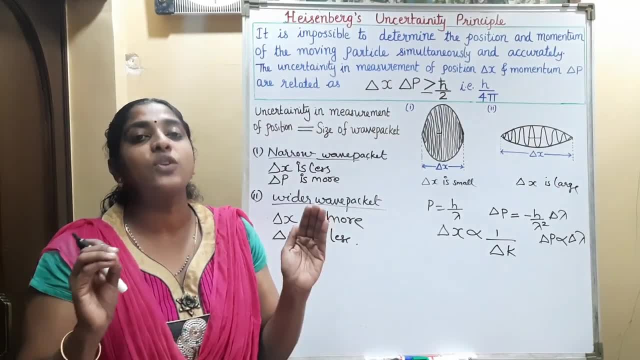 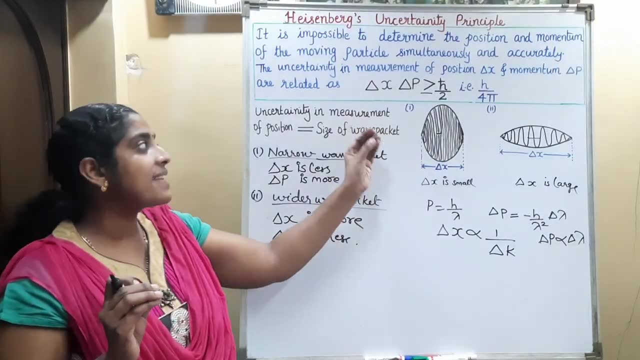 uncertainty. product of these pairs of variables is of the order of planck's constant. where h is planck's constant, h cross is h by 2 pi. so delta x, delta p greater or equal to h cross by 2, that is equal to h by 4 pi. 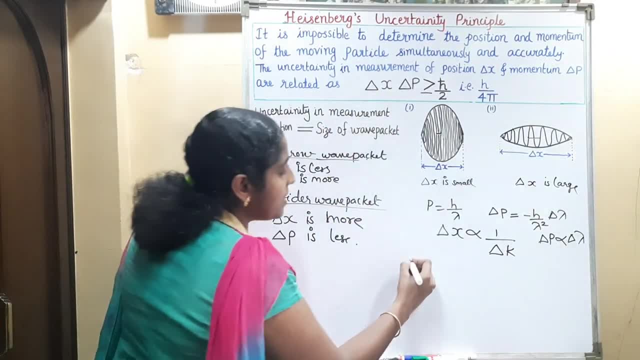 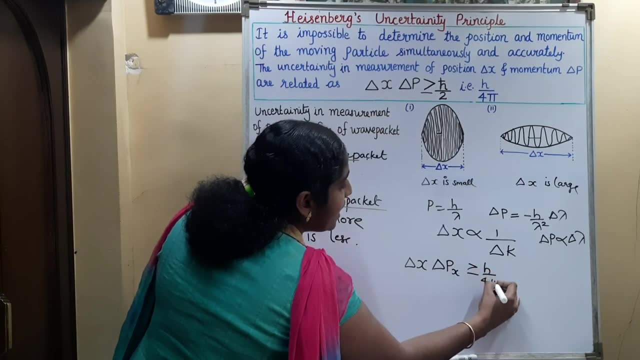 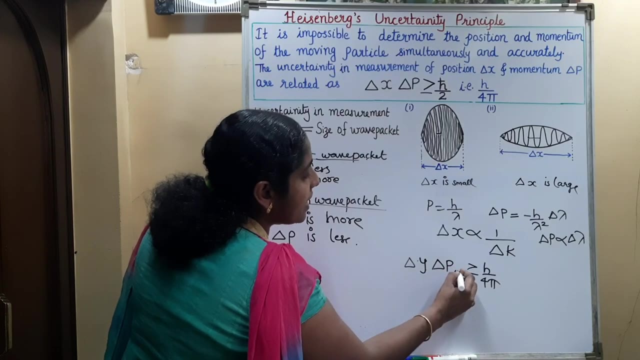 Here the particle is moving along the x direction, So that means delta x. exactly, it is delta x. delta p x greater than or equal to h by 4 pi. If we are taking the motion along the y direction, this will be delta y. delta p y will be greater than or equal to h by 4 pi. 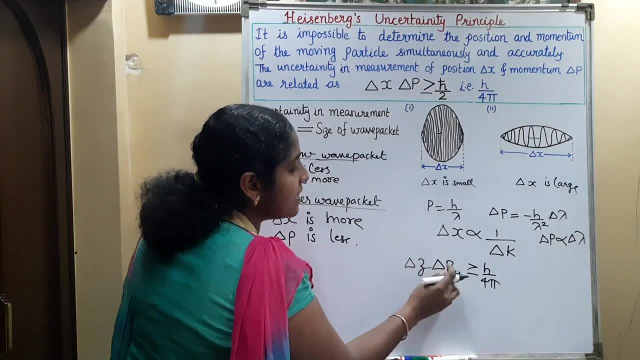 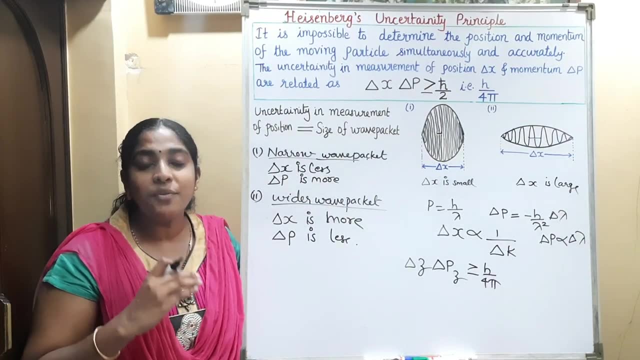 If it is along the z direction, this will be delta z, delta p, z greater than or equal to h by 4 pi. Thus, a wave packet picture is given to a moving particle in such a way that the size of the wave packet is determined by the uncertainty principle. 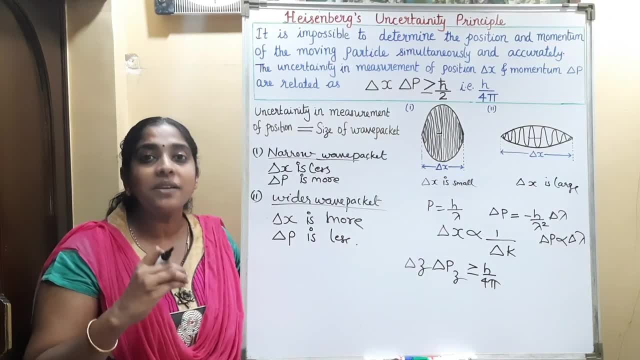 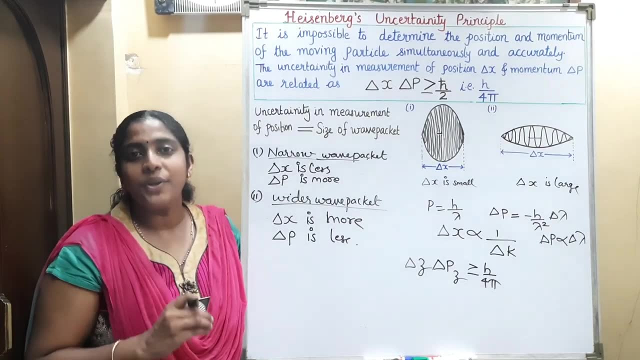 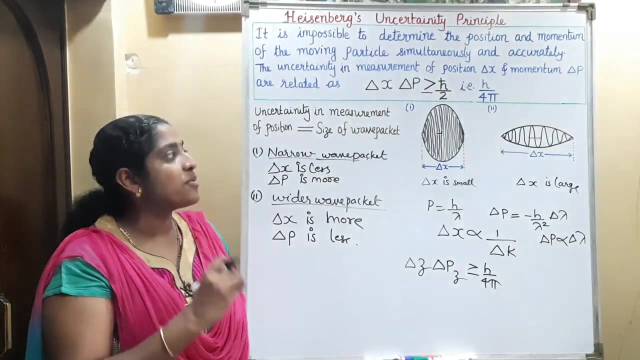 That means the position and momentum can be determined with an accuracy up to the limit that the uncertainty principle allows. So according to Heisenberg's uncertainty principle, whatever may be the accuracy of the instruments we are using to find out the position and momentum of the particle, 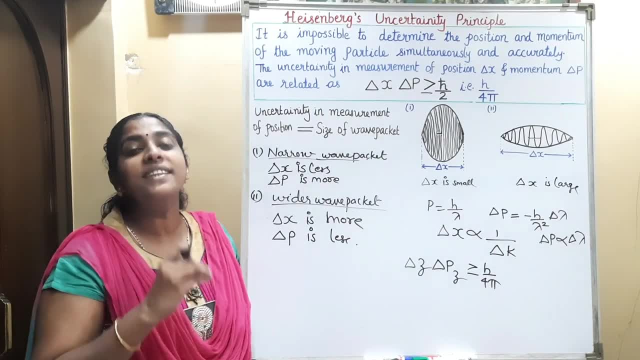 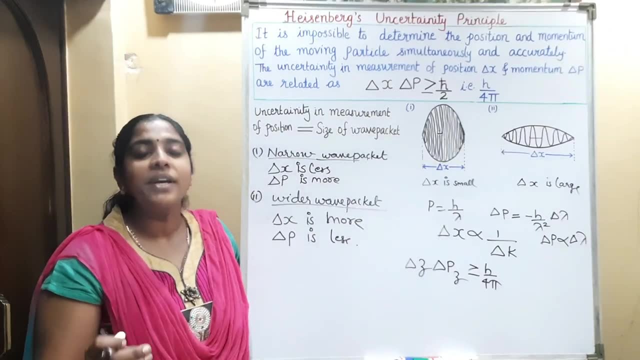 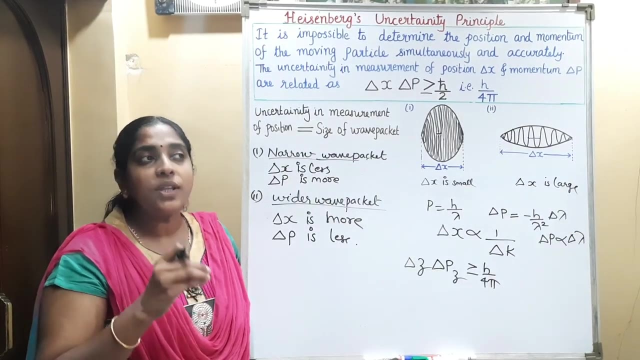 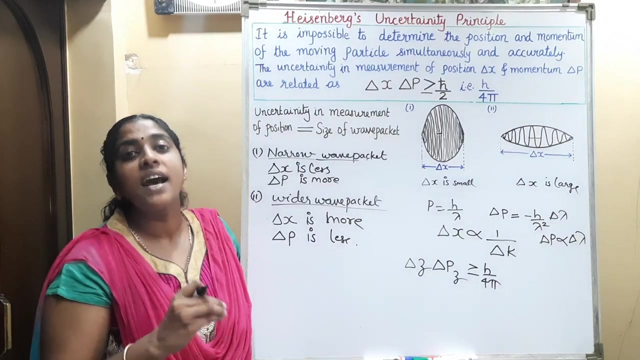 The precision Of that measurement will be within the limit of the Heisenberg's uncertainty principle allows Not only the position and momentum. there are other pairs in the quantum mechanics also which follows this Heisenberg's uncertainty principle. So the pair of variables which follows Heisenberg's uncertainty principle are known as canonically conjugate variables. 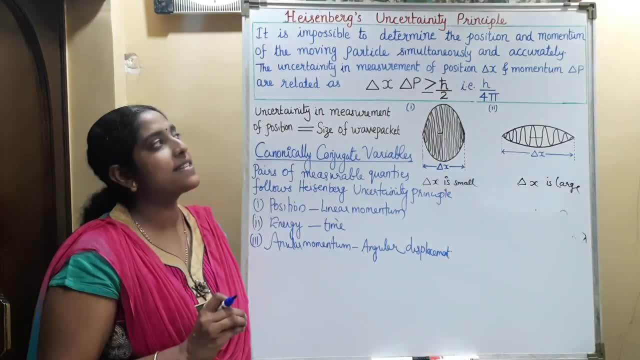 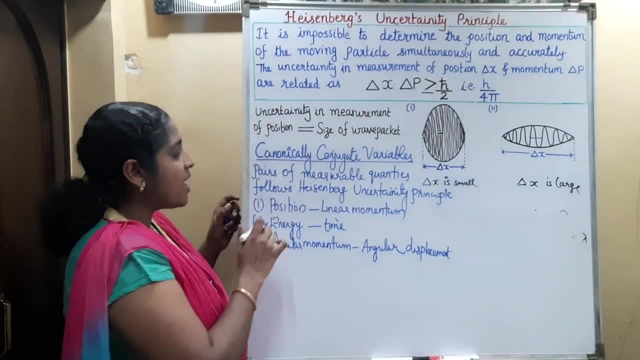 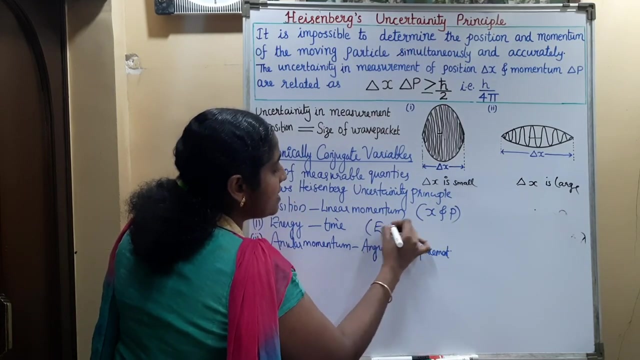 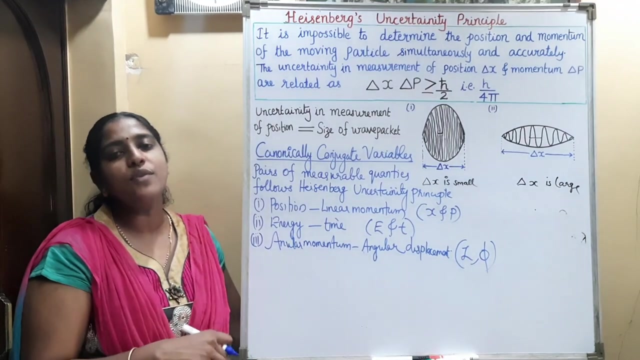 So the pairs of measurable quantities That follows this Heisenberg's uncertainty principles are called canonically conjugate variables. They are position, linear momentum, x and p, energy and time, e and t, and angular momentum and angular displacement, l and phi. They also follows this Heisenberg's uncertainty principles. 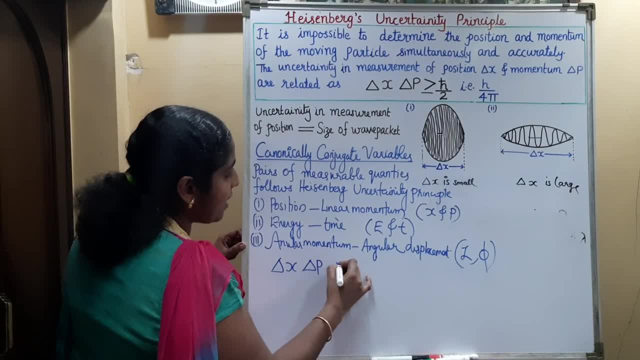 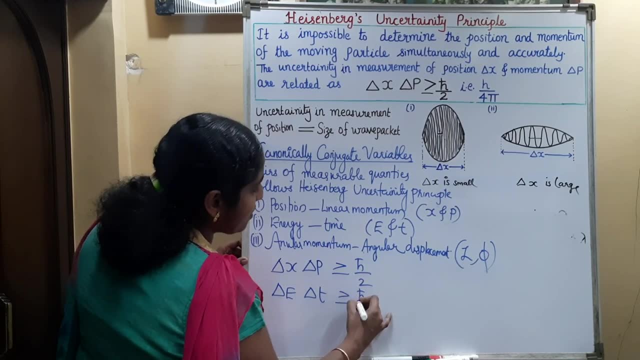 So in that is delta s, delta p, greater than or equal to h, cross by 2.. Delta e, delta t is greater than or equal to h, cross by 2.. Delta l, delta phi, is greater than or equal to h, cross by 2.. 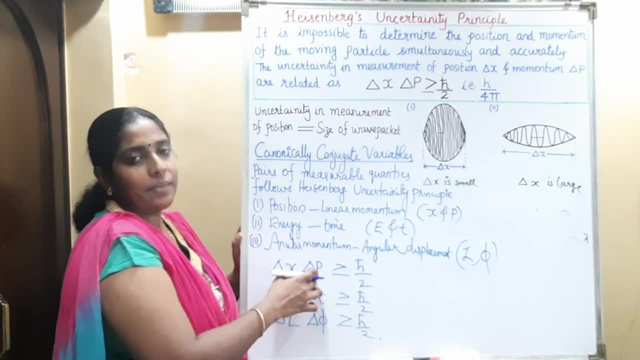 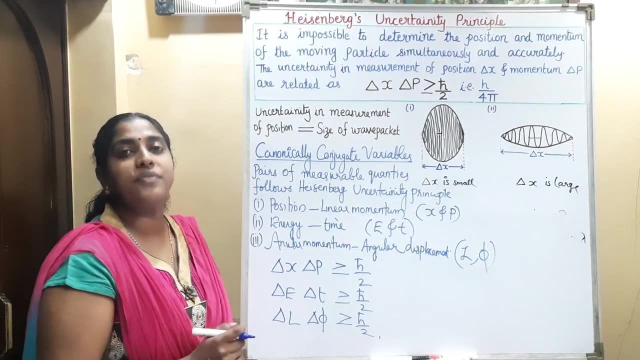 Delta x is the uncertainty in finding the position. Delta p is the uncertainty in finding the momentum. Similarly, delta e is the uncertainty in finding the energy. Delta t is uncertainty in finding the time. Now we can find out the energy. time uncertainty relationship. 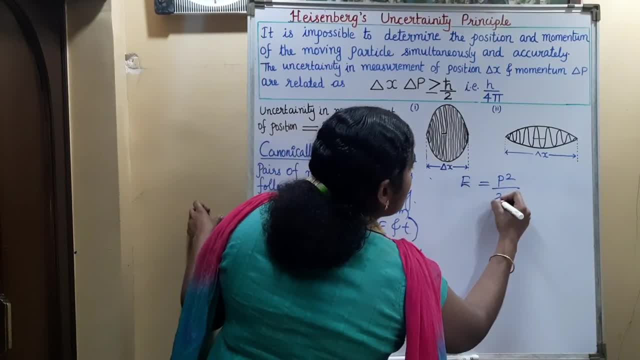 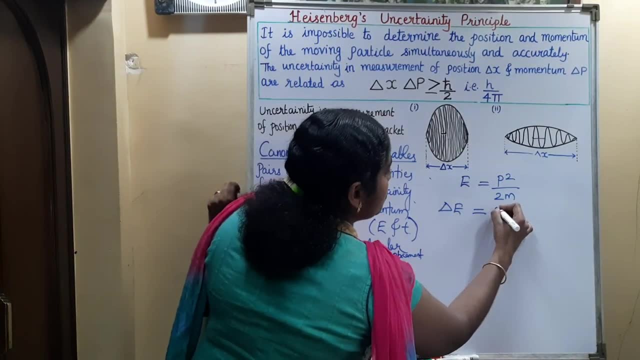 e is equal to p square divided divided by 2m. So if you are taking the uncertainty on both side, This is equal to delta e equal to 2p, delta p divided by 2m. So 2 and 2 will cancel. 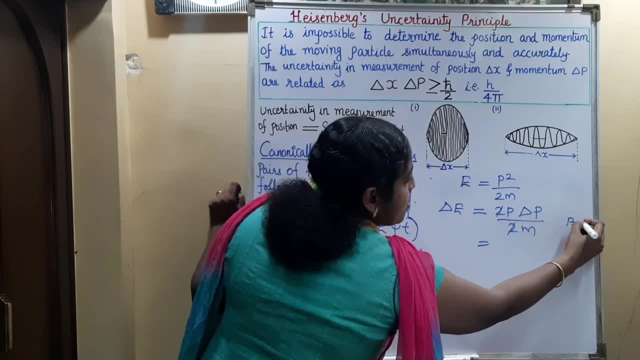 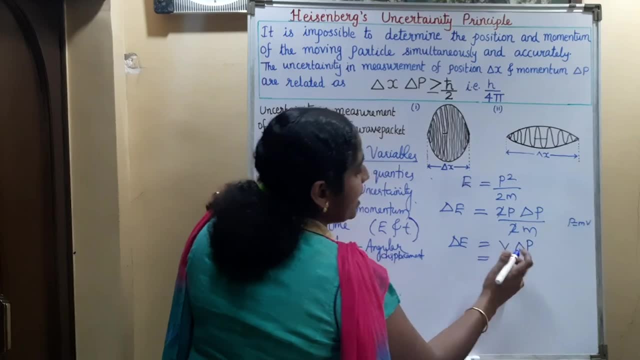 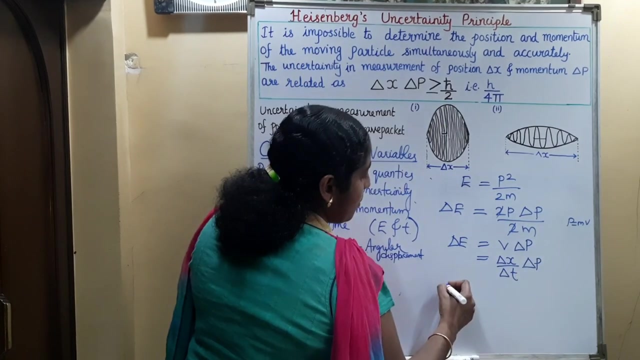 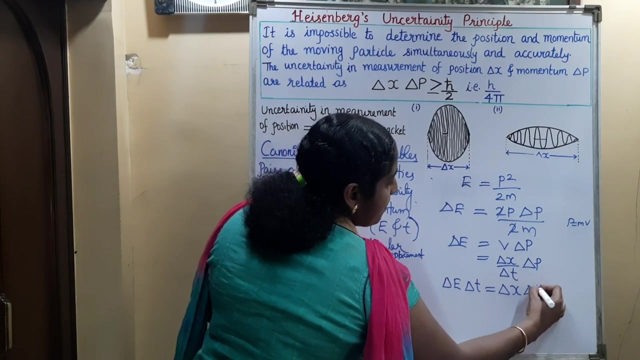 And this p is equal to mv. So m and m will cancel and we are getting v. delta p is equal to delta e. This v is velocity, that is delta x by delta t Into delta p On cross multiplying we are getting delta e. delta t is equal to delta x, delta p. 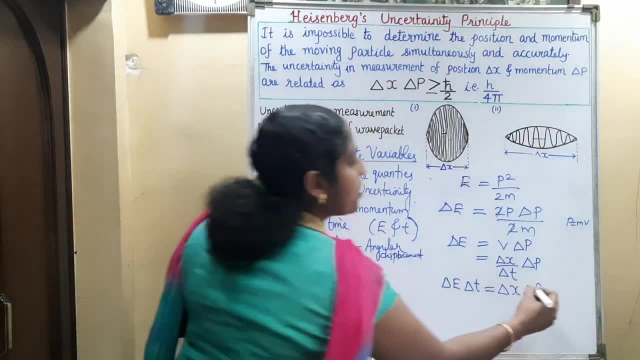 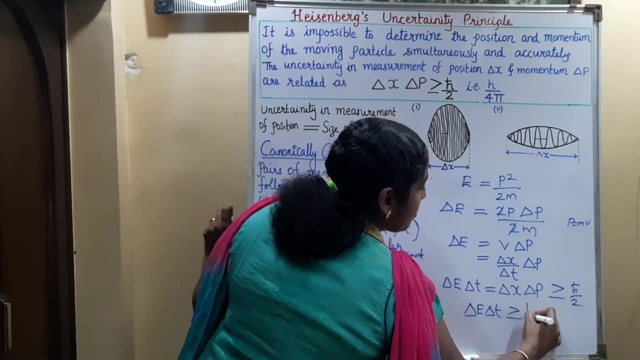 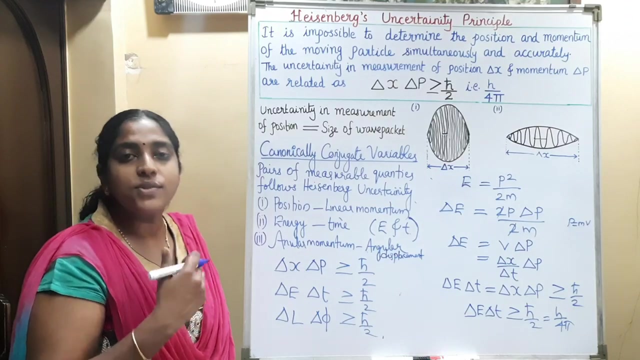 So we know that delta x, delta p is greater than or equal to h cross by 2. That means delta e, delta t is also greater than or equal to h cross by 2. That is h by 4 pi. Therefore energy and time pair also follows Heisenberg's uncertainty principle. 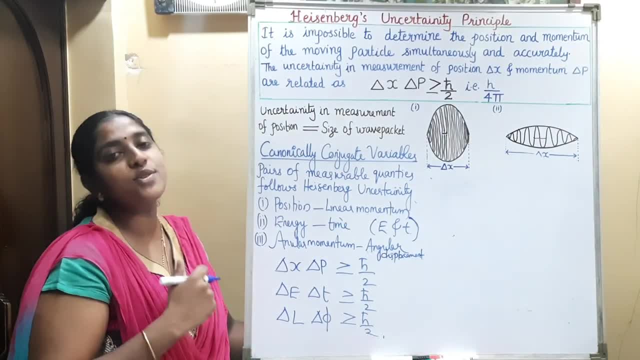 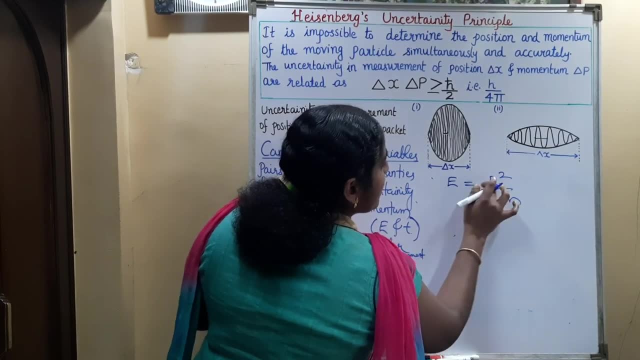 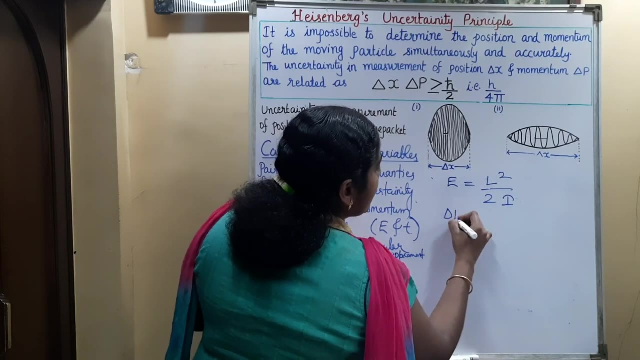 This, similar to this angular momentum and angular displacement, also follows Heisenberg's uncertainty principle. There it was e equal to p, square by 2m. Now we can replace this p by angular momentum l and this m by moment of inertia i. So when we are taking delta e it will be 2l, delta l divided by 2i. 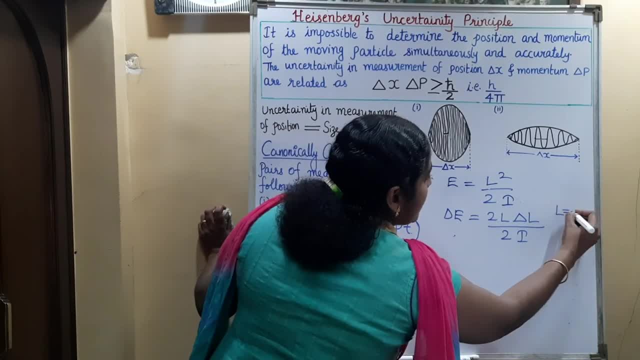 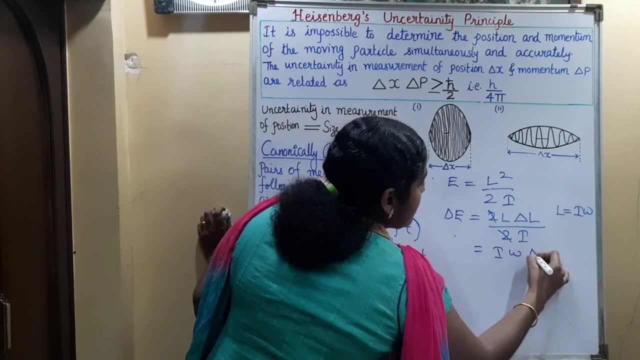 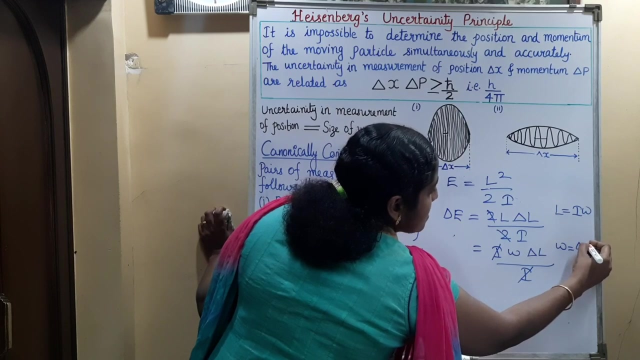 And what is this angular momentum l? Angular momentum l is equal to i- omega. So this is 2, 2 will cancel. and i omega delta l by i And this i i will cancel. And omega is angular velocity, is angular displacement divided by a time interval. 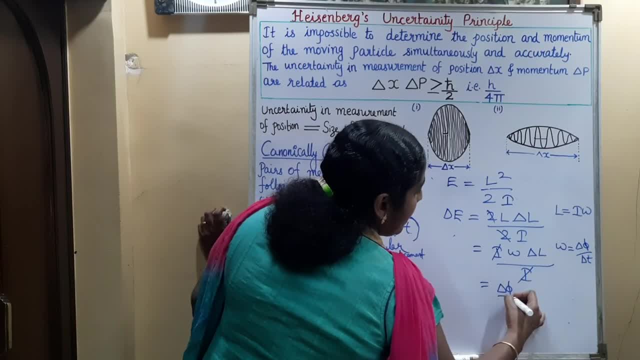 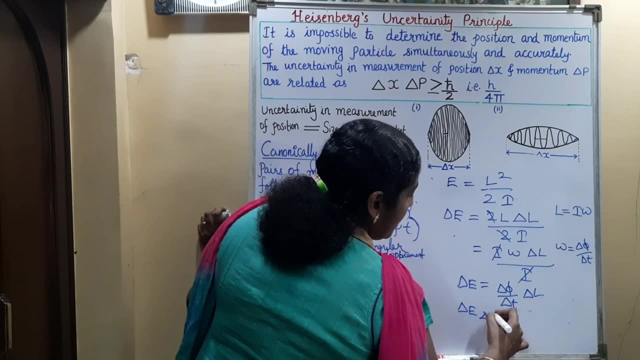 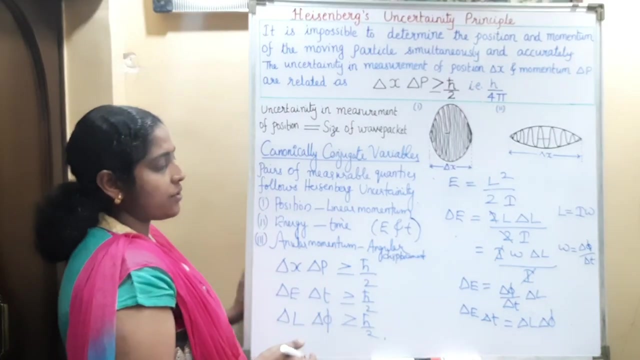 So this will be delta phi, by delta t, delta l, This is delta e. So on cross multiplying, we are getting delta e. delta t is equal to delta l, delta phi, As we know, delta e, So delta t greater than or equal to h, cross by 2.. 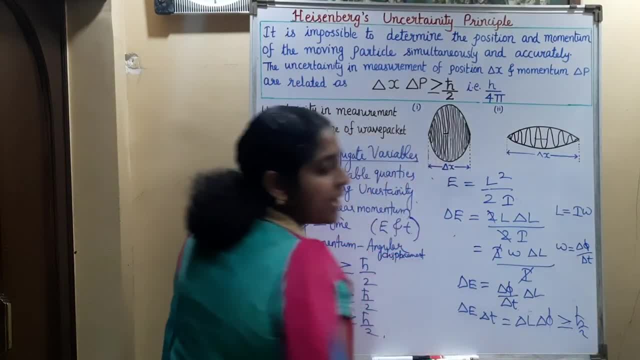 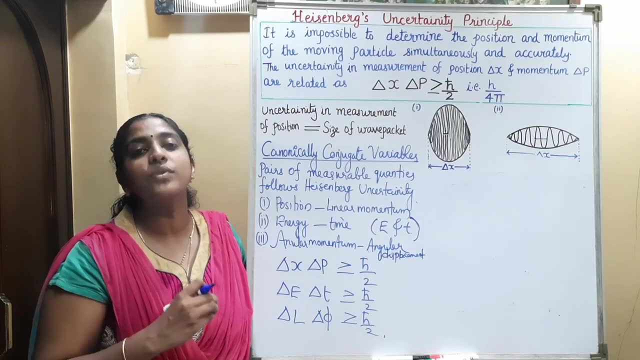 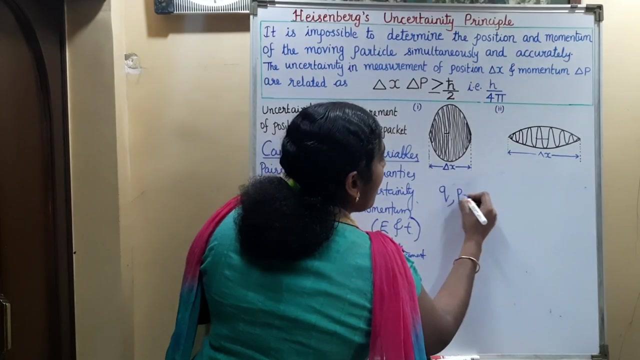 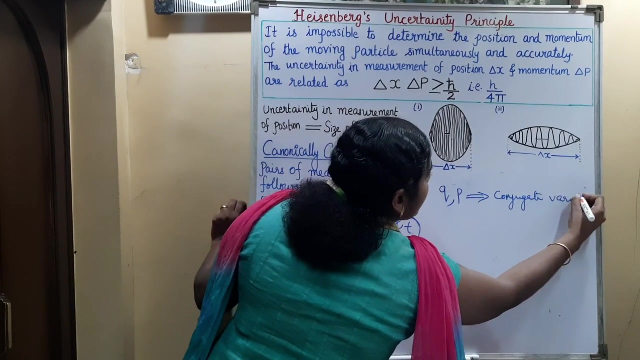 So delta l, delta phi, or also greater than or equal to h, cross by 2.. So Heisenberg's uncertainty principle states that it is impossible to determine two canonically conjugate variables simultaneously and accurately. So if q and p are two conjugate variables, then the Heisenberg's uncertainty relationship we can write it as: